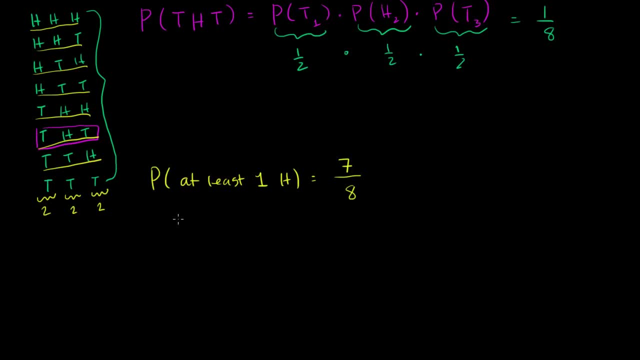 But that would be really hard. if I said at least one head out of 20 flips, This would work well because I only had three flips. So let me make it clear: This is in three flips. This would have been a lot harder to do or more time. 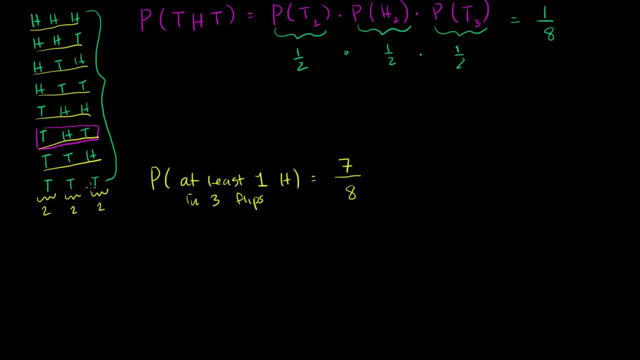 consuming to do if I had 20 flips. Is there some shortcut here? Is there some other way to think about it? And you couldn't just do it in some simple way. You can't just say: oh, probability of heads, times probability of heads. 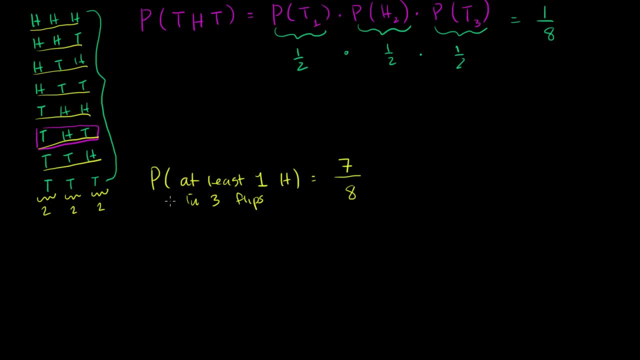 Because if you got heads the first time, then now you don't have to get heads anymore. Or you could get heads again, but you don't have to. So it becomes a little bit more complicated, But there is an easy way to think about it where you could. 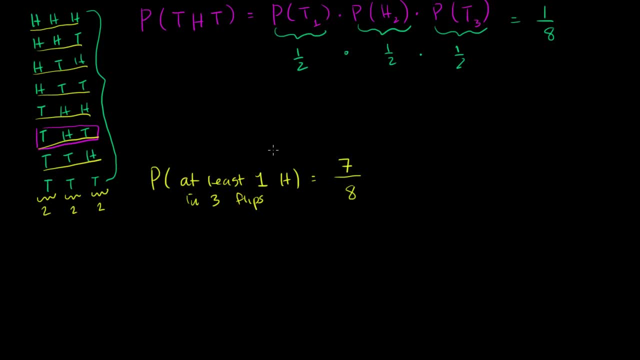 use this methodology right over here. You'll actually see this on a lot of exams where they make it seem like a harder problem. But if you just think about it in the right way, all of a sudden it becomes simpler. One way to think about it is the probability of at least one. 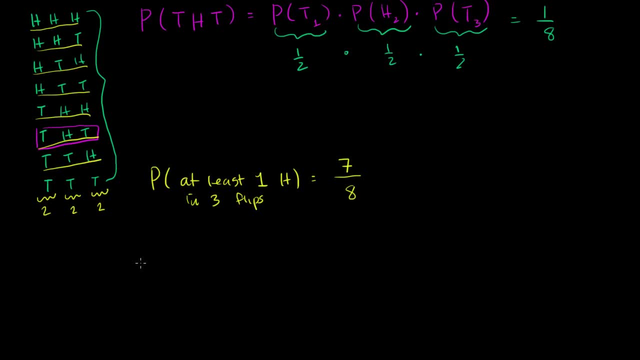 heads in three flips is the same thing as the probability of not getting all tails. If we got all tails, then we would actually don't have at least one head. So these two things are equivalent: The probability of getting at least one head in three flips. 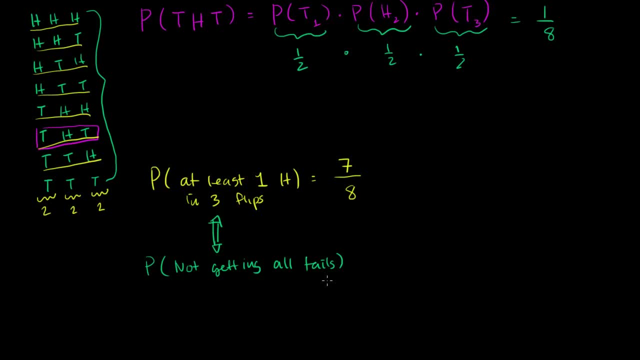 is the same thing as the probability of not getting all tails in three flips. So what's the probability of not getting all tails? Well, that's going to be 1 minus the probability of getting all tails And since it's three flips, it's the probability. 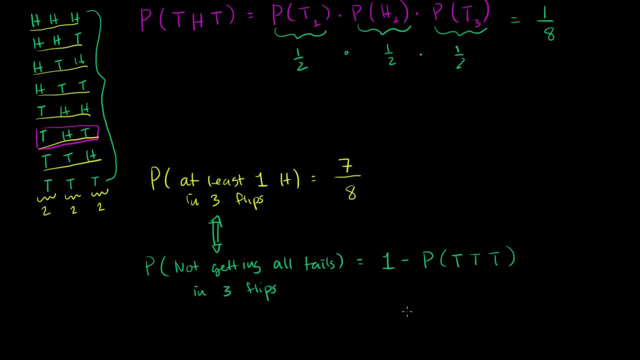 of tails, tails and tails, Because any of the other situations are going to have at least one head in them. And that's all of the other possibilities, And this is the only other leftover possibility. If you add them together, you're going to get one. 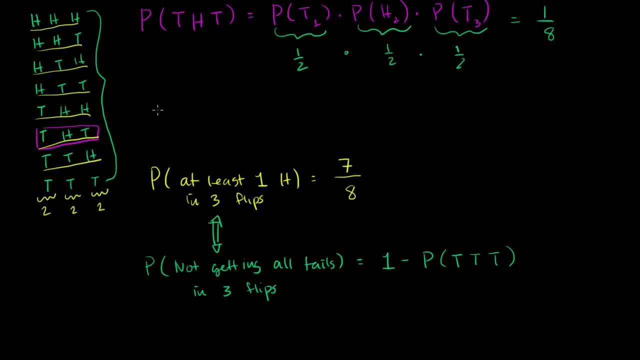 Let me write it this way- The probability- let me write it in a new color, just so you see where this is coming from- The probability of not all tails. not all tails, plus the probability of hailing from the other side of the field. 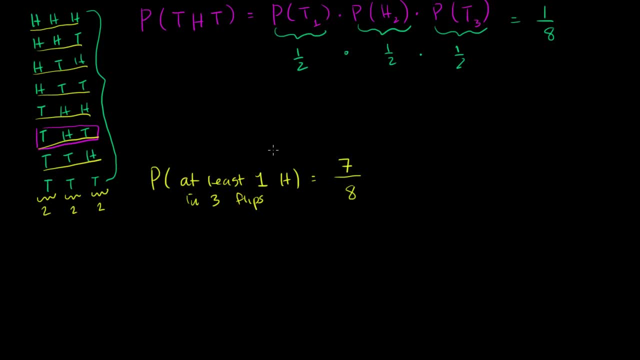 use this methodology right over here. You'll actually see this on a lot of exams where they make it seem like a harder problem. But if you just think about it in the right way, all of a sudden it becomes simpler. One way to think about it is the probability of at least one. 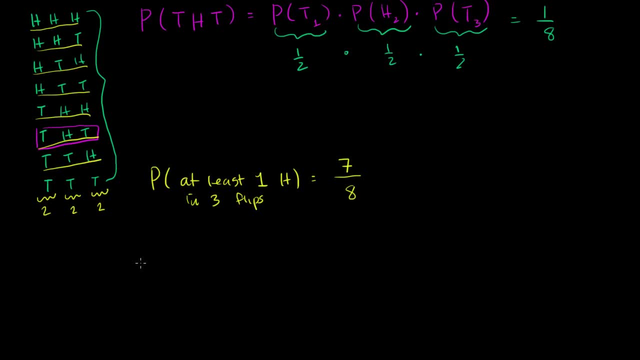 heads in three flips is the same thing as the probability of not getting all tails. If we got all tails, then we would actually don't have at least one head. So these two things are equivalent: The probability of getting at least one head in three flips. 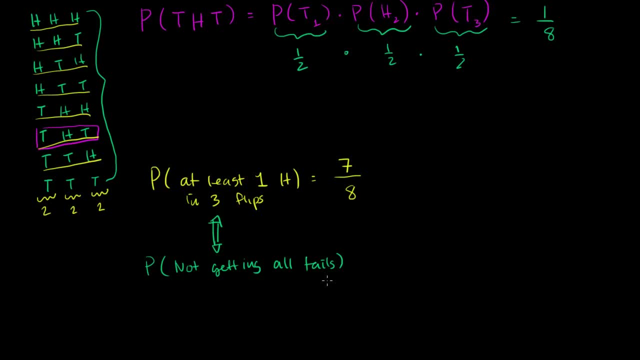 is the same thing as the probability of not getting all tails in three flips. So what's the probability of not getting all tails? Well, that's going to be 1 minus the probability of getting all tails And since it's three flips, it's the probability. 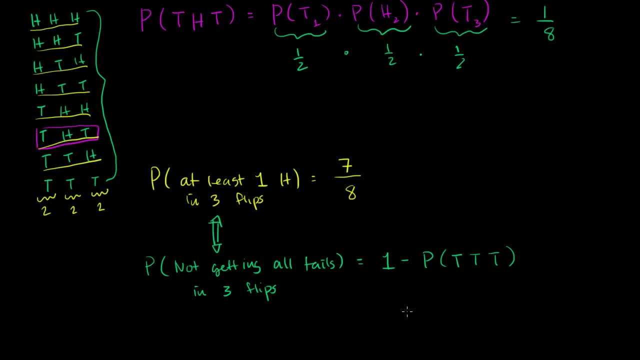 of tails, tails and tails, Because any of the other situations are going to have at least one head in them. And that's all of the other possibilities, and then this is the only other leftover possibility. If you add them together, you're going to get 1.. 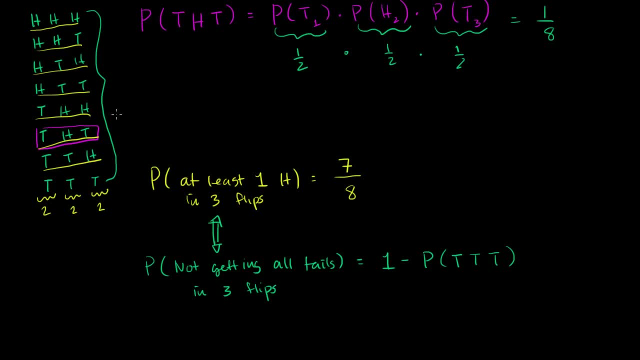 Let me write it this way: The probability- let me write it in a new color, just so you see where this is coming from- The probability of not all tails, not all tails, plus the probability of losing probability of all tails. well, this is essentially exhaustive. 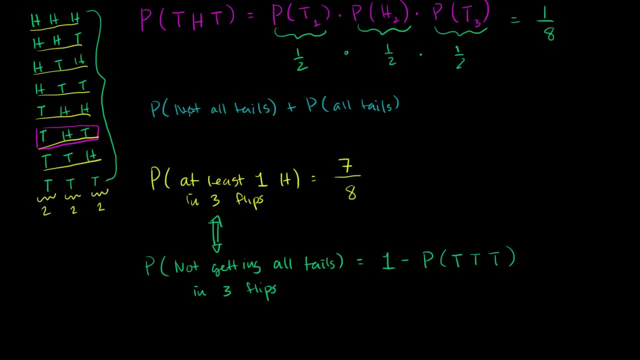 This is all of the possible circumstances. So your chances of getting either not all tails or all tails- and these are mutually exclusive, so we can add them. So the probability of- let me write it this way- the probability of not all tails- or just to be clear what- 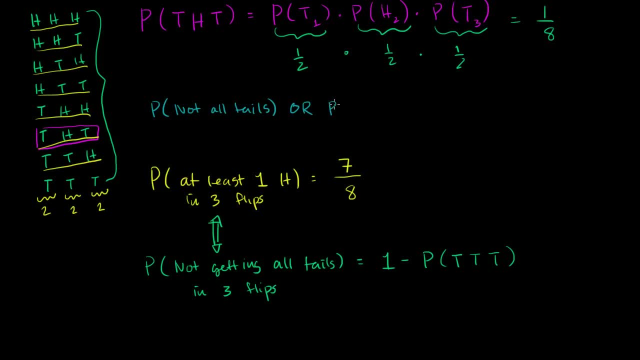 we're doing. the probability of not all tails or the probability of all tails is going to be equal to 1.. These are mutually exclusive. You're either going to have not all tails, which means a head shows up, or you're going to have all tails. 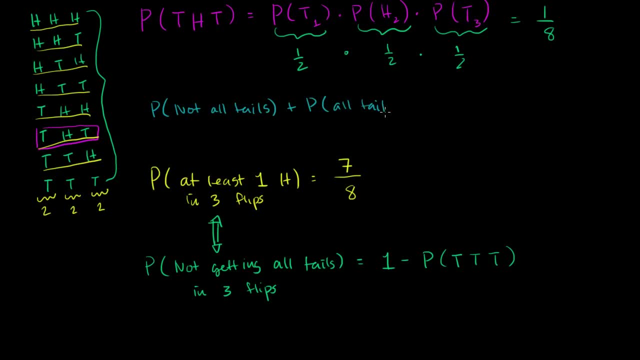 of all tails. well, this is essentially exhaustive. This is all of the possible circumstances, So your chances of getting either not all tails or all tails, and these are mutually exclusive so we can add them. So the probability of- let me write it this way- 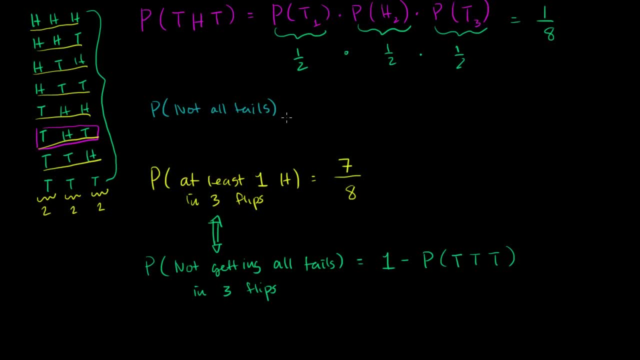 the probability of not all tails or, just to be clear what we're doing, the probability of not all tails or the probability of all tails is going to be equal to 1.. These are mutually exclusive. You're either going to have not all tails, which 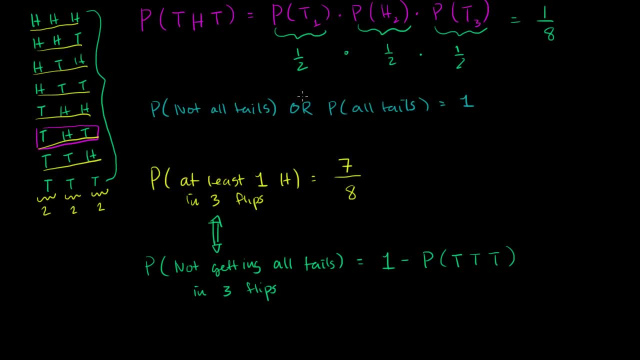 means a head shows up or you're going to have all tails. But you can't have both of these things happening And since they're mutually exclusive and you're saying the probability of this or this happening, you can add their probabilities. 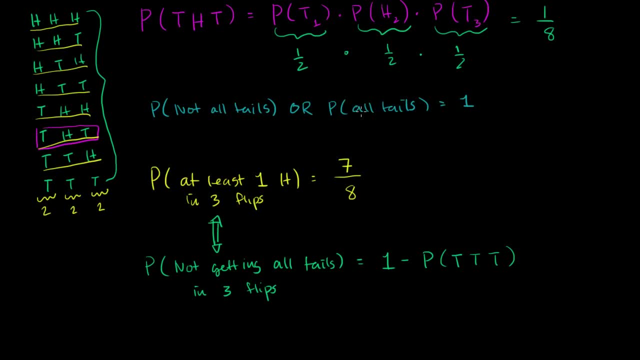 And this is essentially all of the possible events, So all of the probability of it. So So this is essentially, if you combine these, this is the probability of any of the events happening, And that's going to be a 1, or 100% chance. 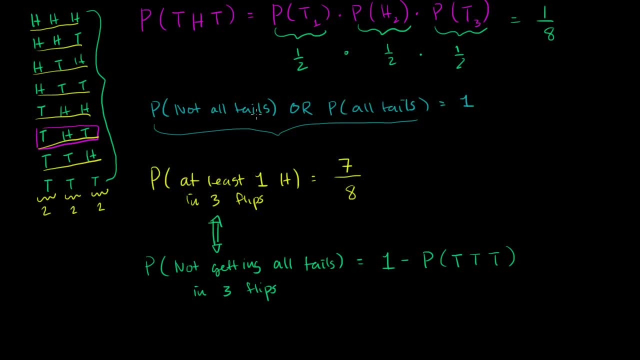 So another way to think about it is: the probability of not all tails is going to be 1 minus the probability of all tails. So that's what we did right over here And the probability of all tails is pretty straightforward. That's the probability of it's going. 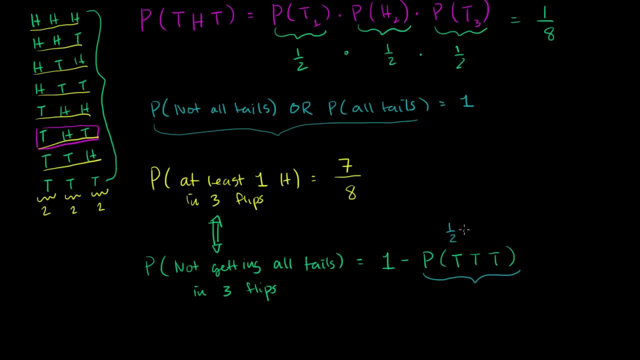 to be 1 half, because you have a 1 half chance of getting a tails on the first flip times. let me write it here. So this is going to be 1 minus the probability of getting all tails. well, you have a 1 half chance of getting tails. 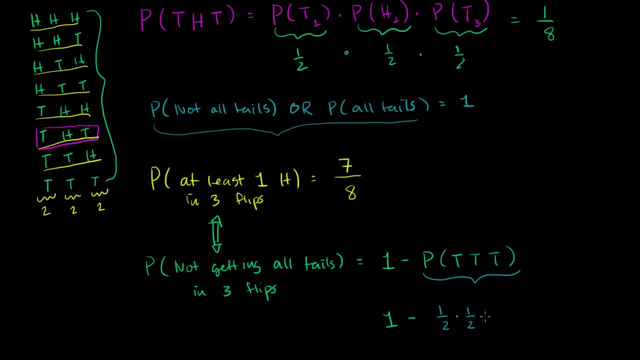 on the first flip, and then you're going to have to get another tails on the second flip, and then you're going to have to get another tails on the third flip, And then 1 half times 1 half times, 1 half. 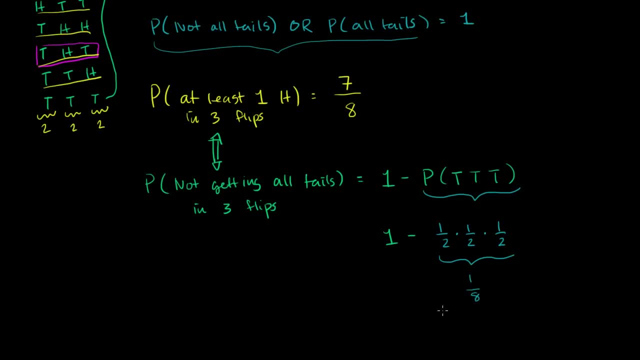 this is going to be 1 eighth, And then 1 minus 1 eighth or 8 eighths minus 1 eighth is going to be equal to 7 eighths. So Let's apply that to a problem that. 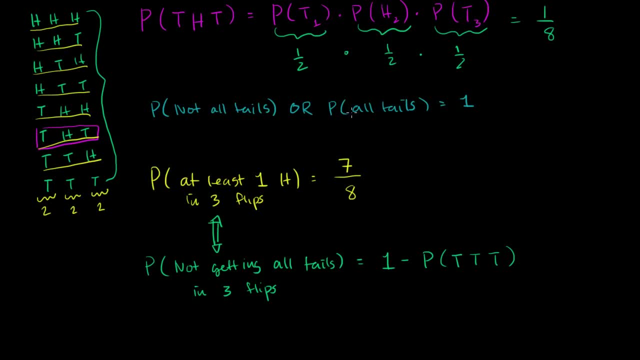 But you can't have both of these things happening And since they're mutually exclusive and you're saying the probability of this or this happening, you can add their probabilities And this is essentially all of the possible events. So this is essentially, if you 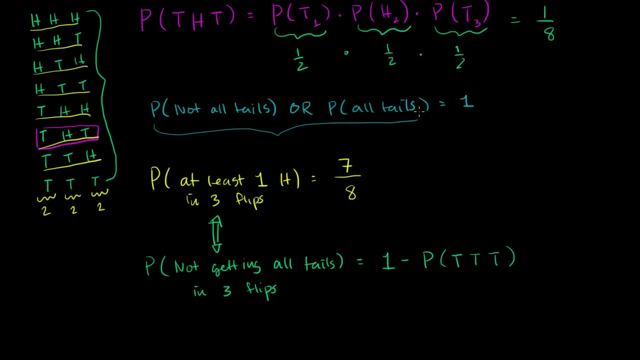 come up with the probability of not all tails or all tails and you combine these. this is the probability of any of the events happening, And that's going to be a 1, or 100% chance. So another way to think about it is the probability of not. 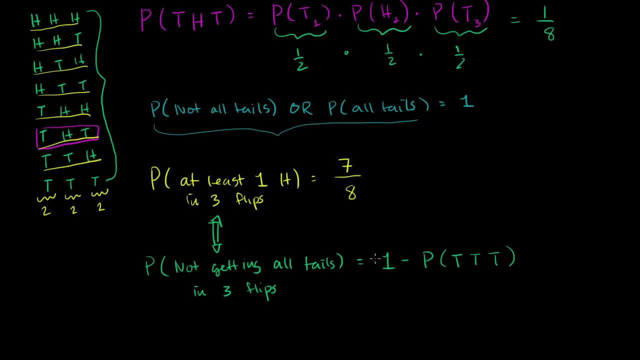 all tails is going to be 1 minus the probability of all tails. So that's what we did right over here And the probability of all tails is pretty straightforward. That's the probability of it's going to be 1 half, because you have a 1 half chance of getting a tails on the first. 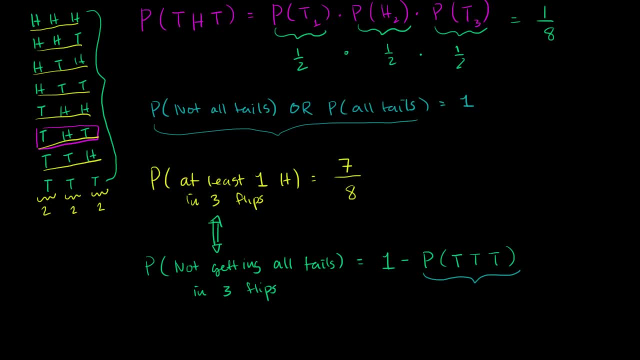 flip times. let me write it here so it becomes a little clearer. So this is going to be 1 minus the probability of getting all tails. Well, you have a 1 half chance of getting tails on the first flip and then you're going to have to get another tails on. 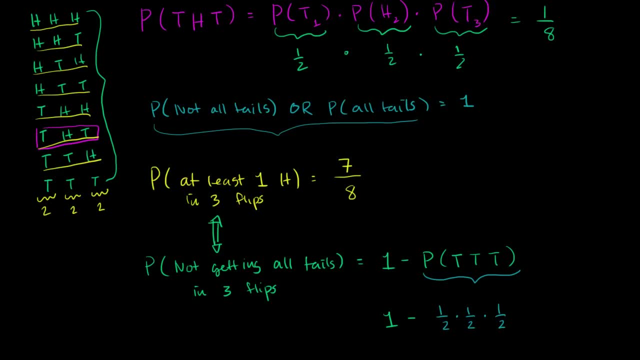 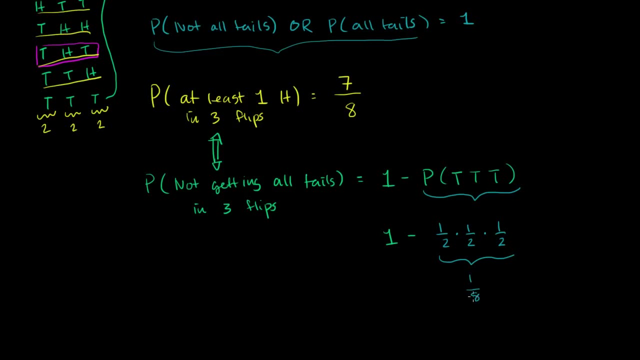 the second flip, and then you're going to have to get another tails on the third flip, And then 1 half times 1 half times 1 half. this is going to be 1 eighth, And then 1 minus 1 eighth, or 8 eighths minus 1 eighth is. 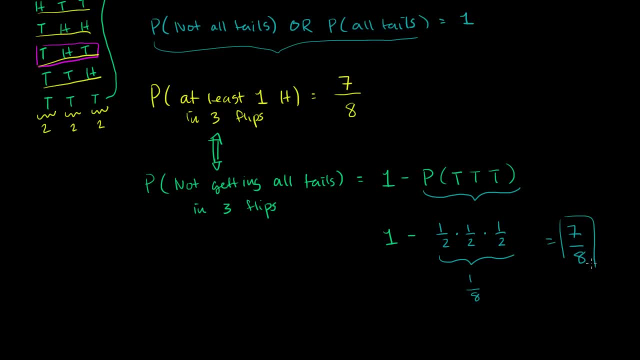 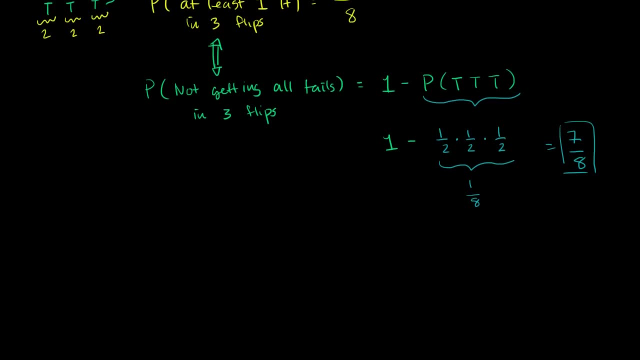 going to be equal to 7 eighths. So we can apply that to a problem that is harder to solve than writing all of the scenarios like we did in the first problem. We can say: let's say we have 10 flips. 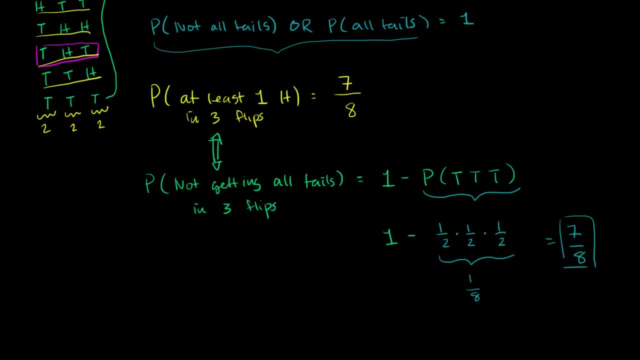 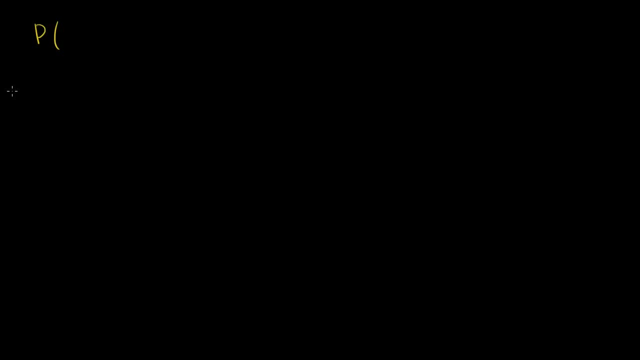 is harder to do than writing all of the scenarios like we did in the first problem. We can say: let's say we have 10 flips. The probability of at least 1 head in 10 flips. Well, we use the same idea. 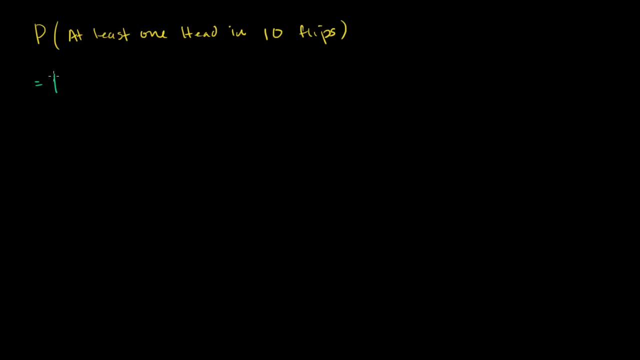 This is the same thing. This is going to be equal to the probability of not all tails in 10 flips. So we're just saying the probability of not getting all of the flips going to be tails. All of the flips is tails, Not all tails in 10 flips. 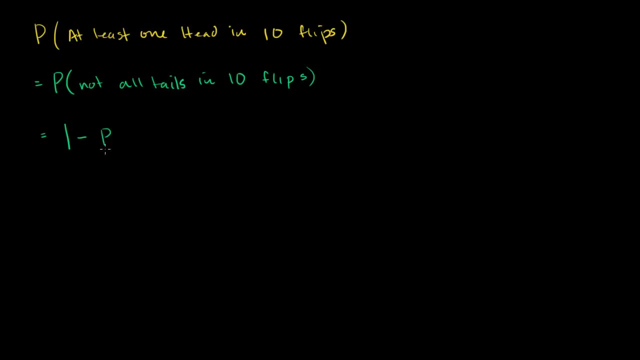 And this is going to be 1 minus the probability of flipping tails 10 times. So it's 1 minus 10 tails in a row, 10 tails in a row, And so this is going to be equal to this part right over here. 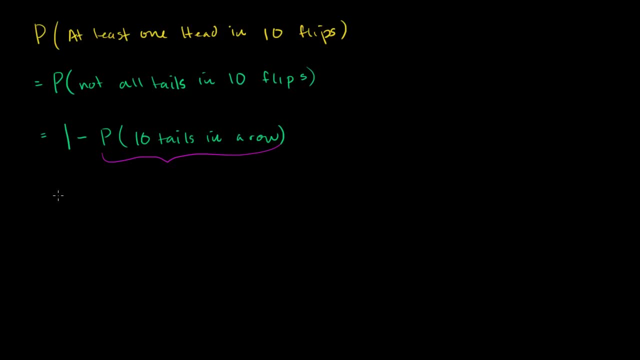 Let me write this. So this is going to be this 1.. Let me just rewrite it. This is equal to 1 minus And this part is going to be: well, 1 tail, another tail, So it's 1 half times 1 half. 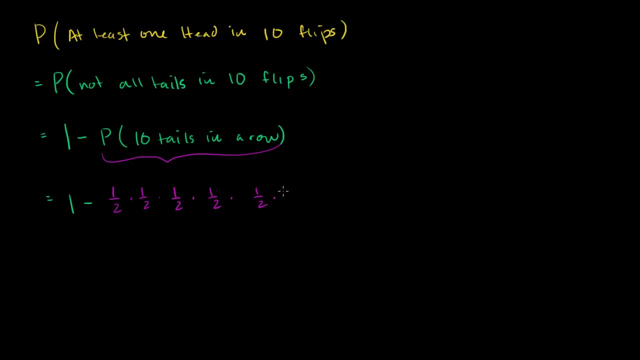 And I'm going to do this 10 times. I'm going to do this 10 times. Let me write this a little neater, because I need a 1 half. So that's 5., 6., 7., 8.. 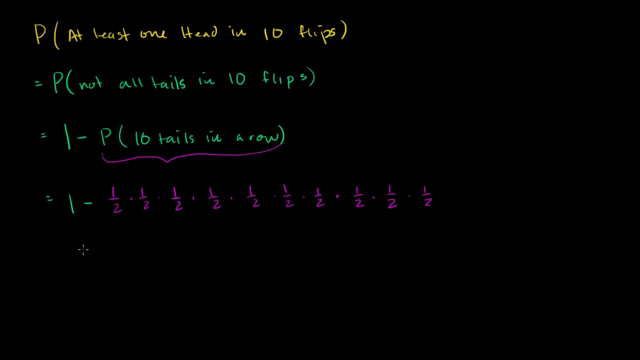 9. And 10.. And so we really just have to. the numerator is going to be 1.. So this is going to be 1.. This is going to be equal to 1.. Let me do it in that same color of green. 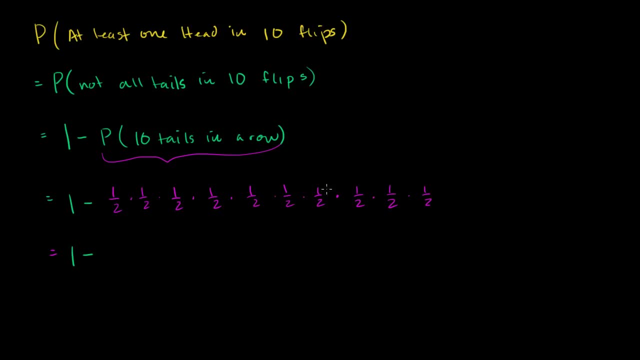 This is going to be equal to 1 minus Our numerator. you just have 1 times itself 10 times, So that's 1.. And then on the denominator you have: 2 times 2 is 4.. 4 times 2 is 8.. 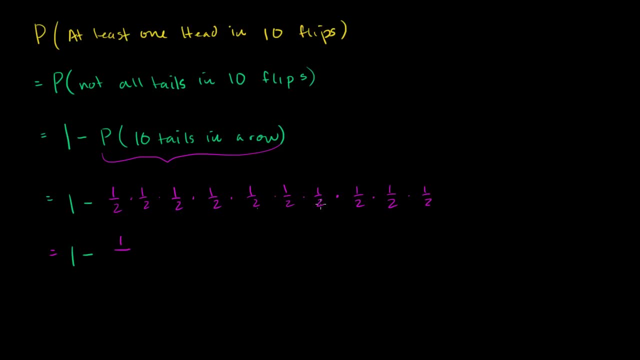 16,, 32,, 64,, 128,, 256,, 512,, 1,024.. Over 1,024.. This is the same, exact same thing as 1 is 1024 over 1024 minus 1.. 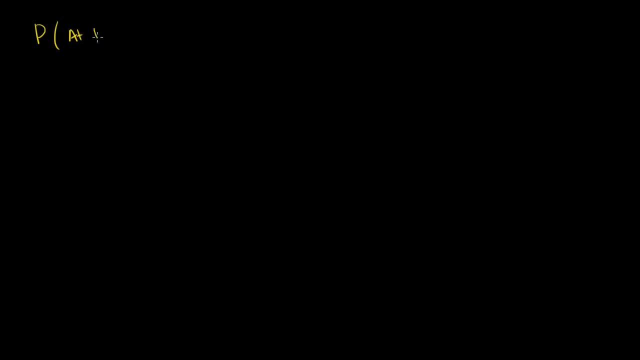 The probability of at least 1 head in 10 flips. Well, we use the same idea. This is the same thing. This is going to be the probability. This is going to be equal to the probability of not all tails in 10 flips. 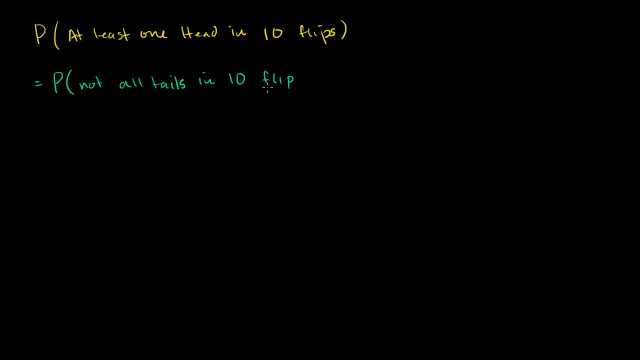 Not all tails. So we're just saying the probability of not getting all of the flips going to be tails. All of the flips is tails, Not all tails in 10 flips And this is going to be 1 minus the probability of flipping. 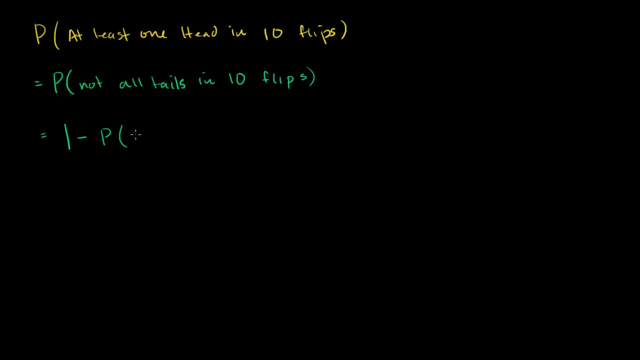 tails 10 times, So it's 1 minus 10 tails in a row, And so this is going to be equal to this part right over here. Let me write this: So this is going to be this 1.. Let me just rewrite it. 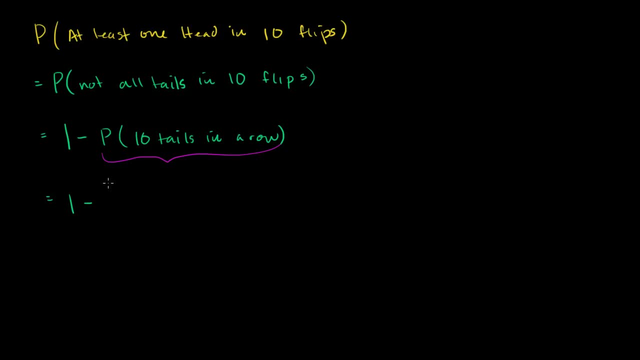 This is equal to 1 minus, And this part is going to be: well, 1 tail, another tail, So it's 1 half times 1 half, And I'm going to do this 10 times. Let me write this a little neater, because I need a 1. 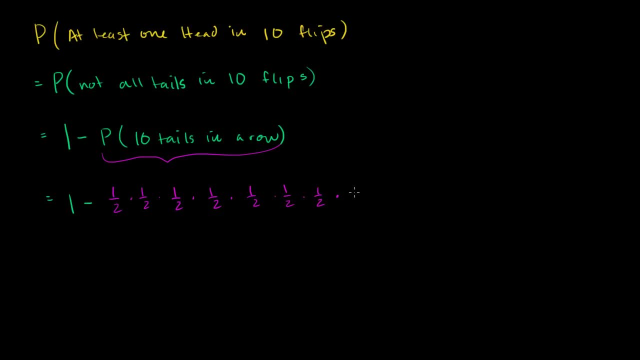 half. So that's 5,, 6,, 7,, 8.. 9, and 10.. And so we really just have to. the numerator is going to be 1.. So this is going to be 1.. This is going to be equal to 1.. 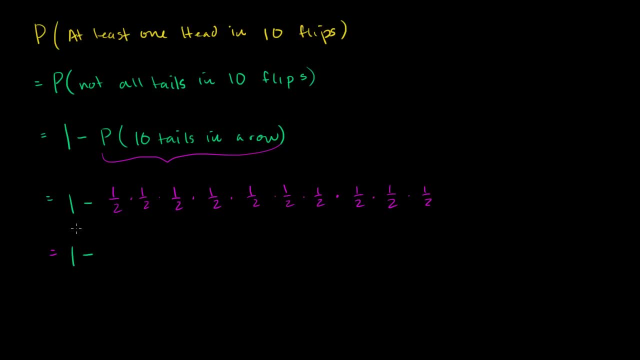 Let me do it in that same color of green. This is going to be equal to 1 minus Our numerator. you just have 1 times itself 10 times, So that's 1.. And then on the denominator, you have 2 times 2 is 4.. 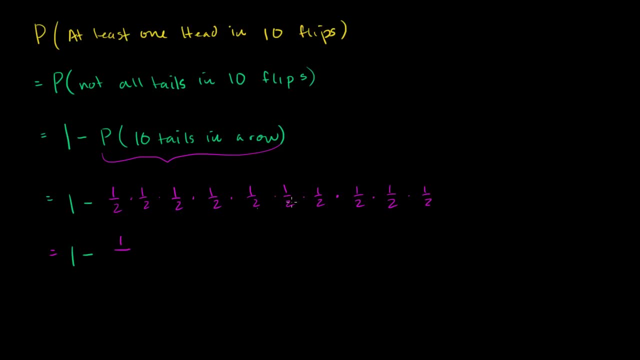 4 times 2 is 8. 16. 32. 64. 128. 256., 512. 1,024.. This is the same exact same thing as 1 is 1024 over 1024, minus 1 over 1024, which is equal to 1023, or 1,023.. 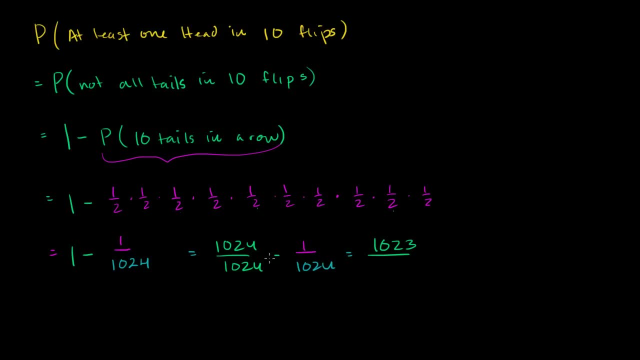 1,023 over 1,024.. We have a common denominator here, So 1,000, I'm doing that same: blue over 1,024.. So if you flip a coin 10 times in a row, a fair coin. 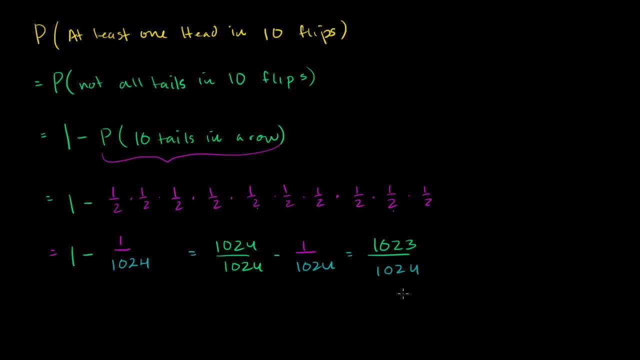 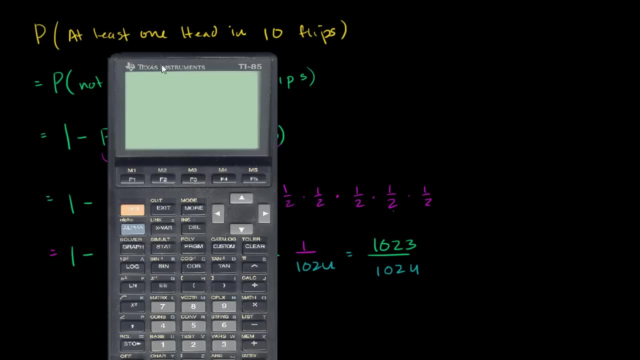 you're probably getting at least 1 heads in that 10 flips. It's pretty high. It's 1,023 over 1,024.. You can get a calculator out to figure that out in terms of a percentage. Actually, let me just do that just for fun. 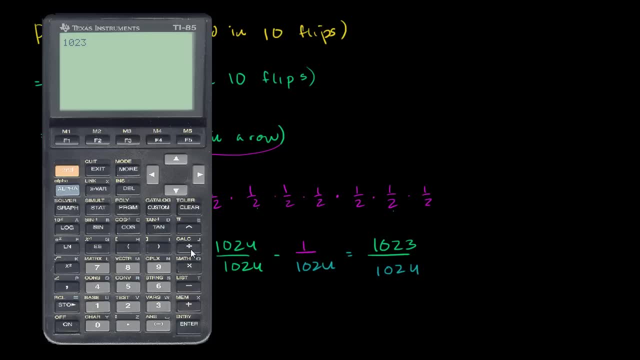 So if we have 1,023 over 1,024.. 1,023 over 1,024.. 1,023 divided by 1,024.. You have a 99.9% chance that you're going to have at least 1 heads. 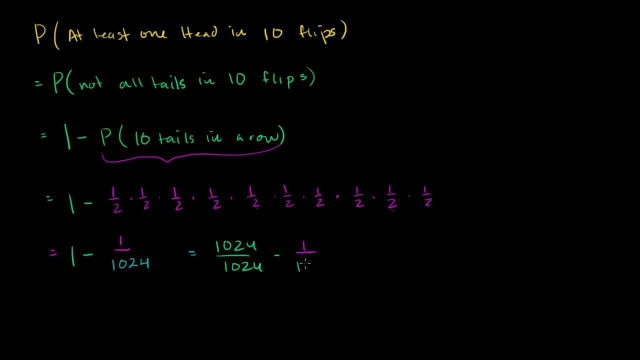 Minus 1 over 1024.. Over 1024.. Which is equal to 1023.. Or 1,024.. 1,024. 1,024. 1,023.. 1,023 over 1,024.. 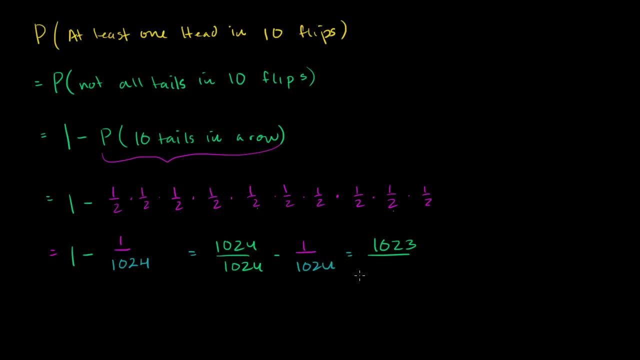 We have a common denominator here, So 1,000.. Doing that same, blue Over 1,024.. So if you flip a coin 10 times in a row- a fair coin- you're probably getting at least one heads in that 10 flips. 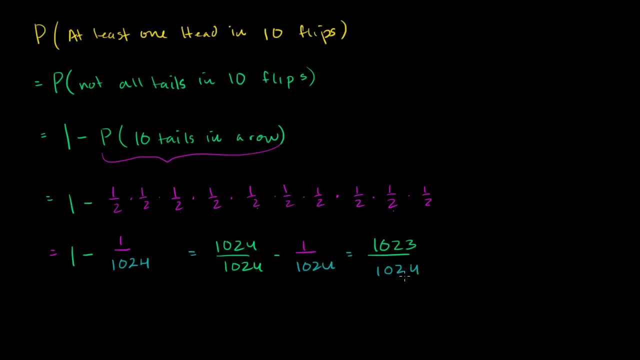 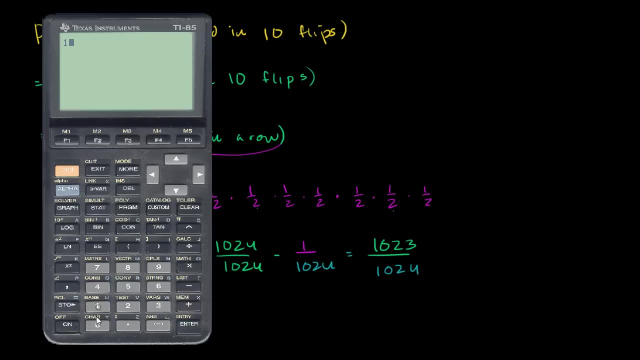 It's pretty high. It's 1,023 over 1,024.. You can get a calculator out to figure that out in terms of a percentage. Actually, let me just do that just for fun. So if we have 1,023 divided by 1,024, you. 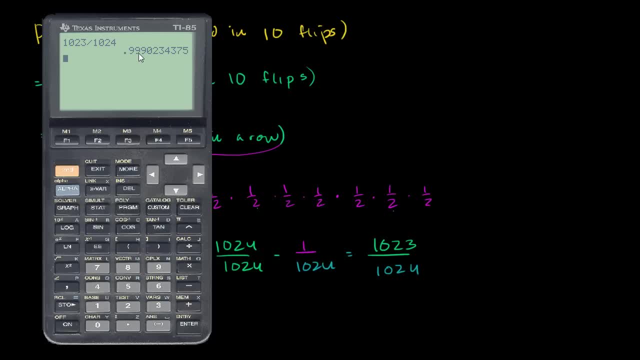 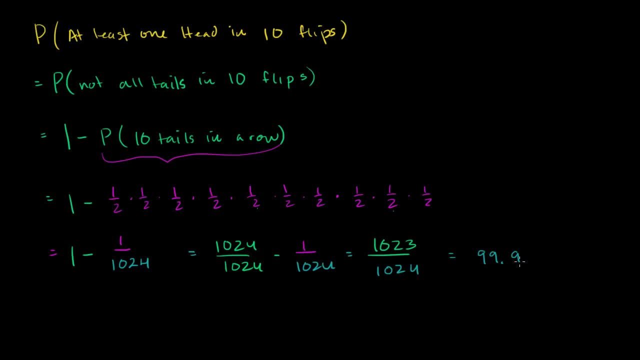 have a 99.9% chance that you're going to have at least one heads. So this is: if we round, this is equal to 99.9% chance, And I rounded a little bit, It's actually even slightly higher than that. 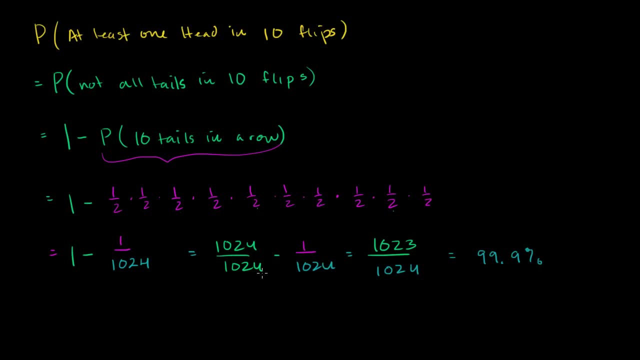 And this is a pretty powerful tool, or a pretty powerful way to think about it, Because it would have taken you forever to write, To write all of the scenarios down. In fact, there would have been 1,024 scenarios to write down. 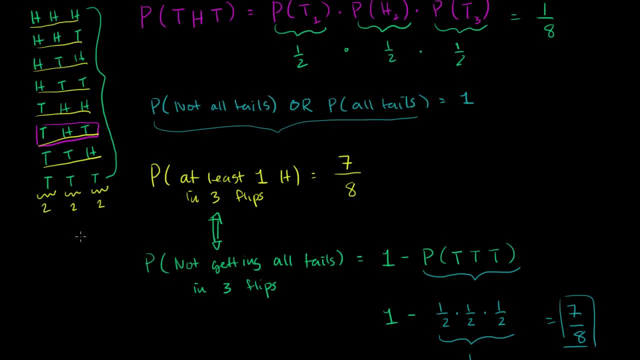 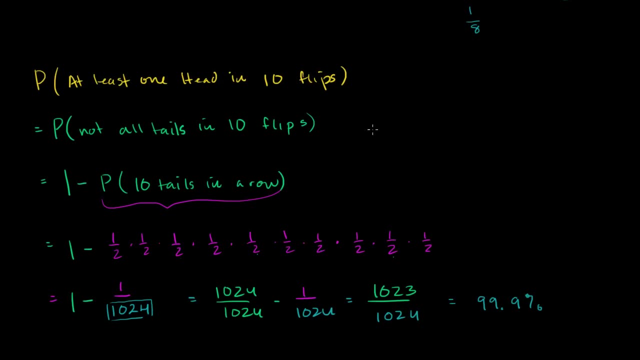 So doing this exercise for 10 flips would have taken up all of our time. But when you think about it in a slightly different way, when you just say, look, the probability of getting at least one heads in 10 flips is the same thing as the probability of not getting.